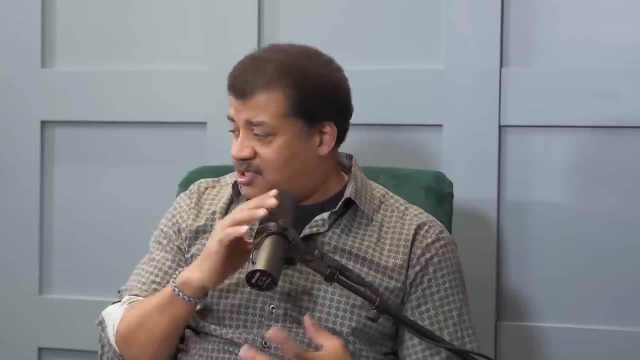 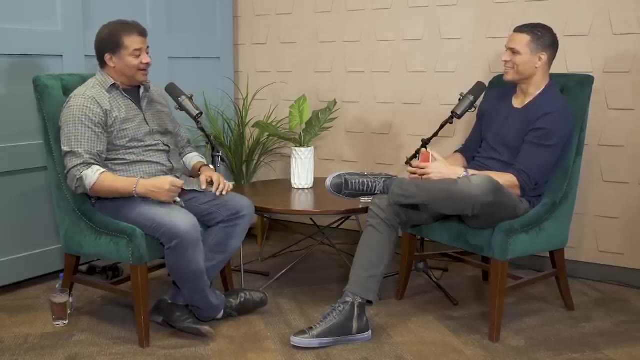 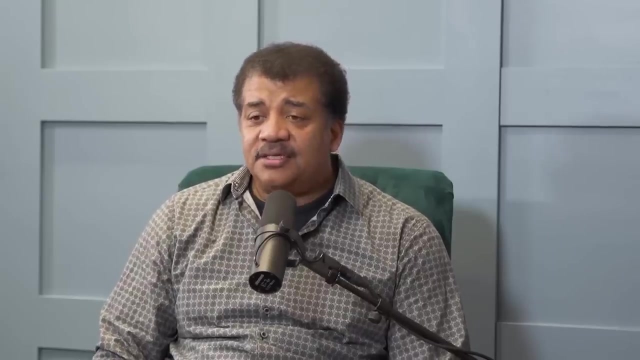 universe is speaking this language. I'm screaming at you. Sorry, The sound levels, Okay, Sorry, Okay. All right, You're excited, This is good, All right. So I said all right, one step at a time. So after the first week of class, 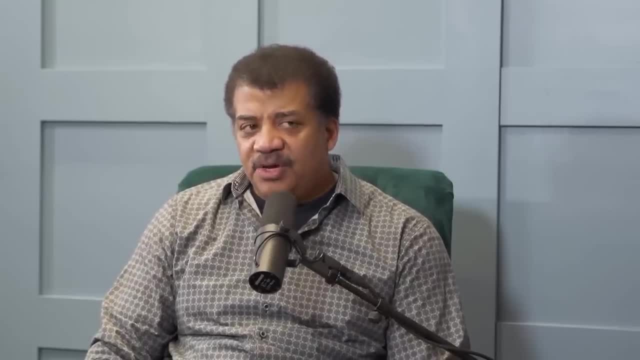 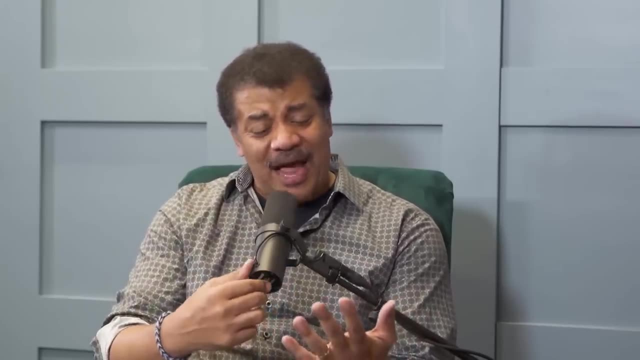 I took a peek: still nothing. After three weeks and a month, open up the side of the book and say, hey, I know that equation, I used that the other day, That's good, I like that. And then, as the 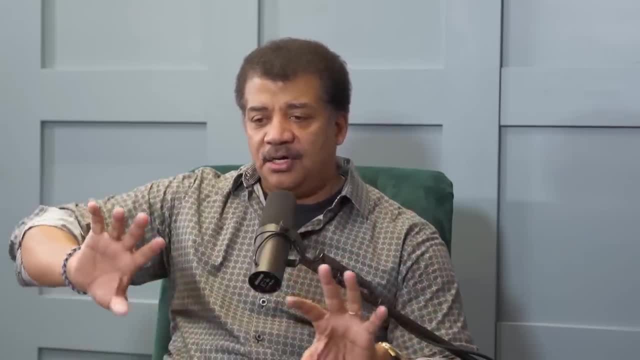 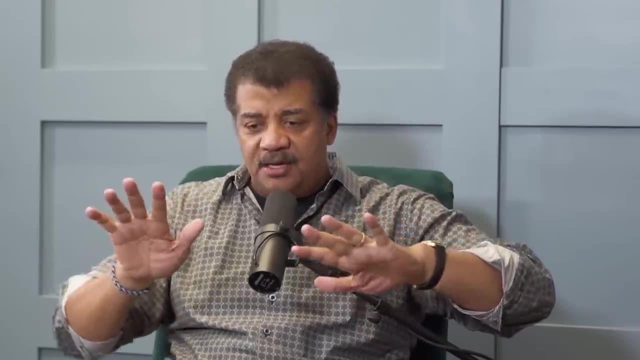 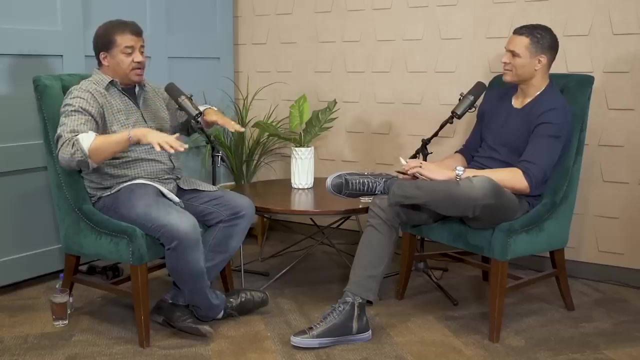 weeks went on. it was as though this fog began to dissipate. It didn't lift, because that implies: now you see it, now you don't, and now you do. It just dissipated. It became more and more transparent And by month three, month four, every one of these equations became my friends. 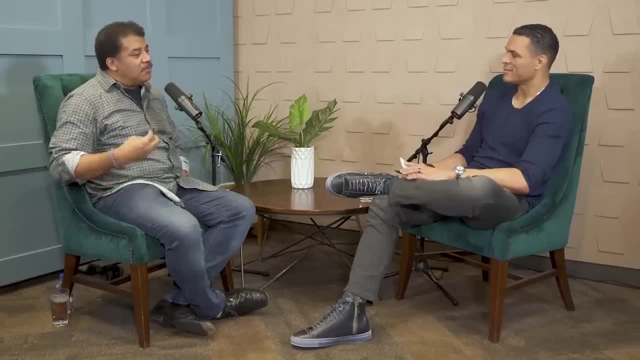 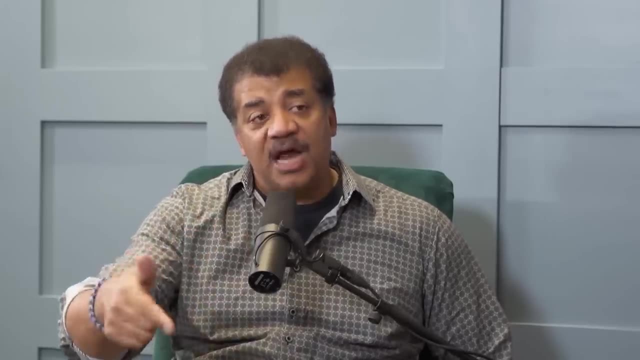 I said I want them. In fact, give me more, And that is my measure of what I need to do if I encounter something which, in that moment, I do not understand. Is that any worse than you coming upon a book of Mandarin? 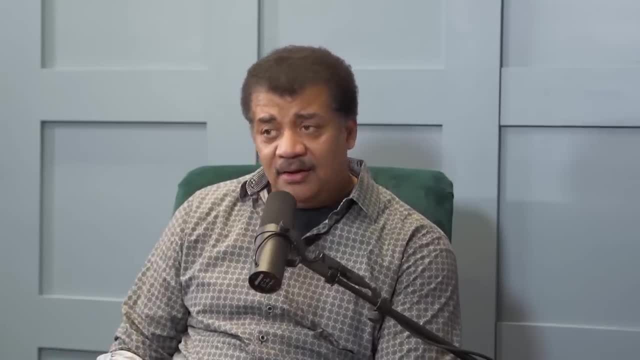 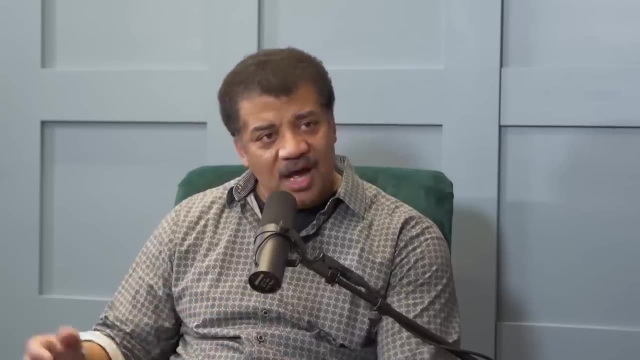 You don't know any Chinese characters. I don't know any of this, Yeah, except one and a half billion people in the world speak it. So it can't be impossible to learn. So you put in the time and slowly, some of the characters. oh, that means a human, or that's a home, or that's a food And all. 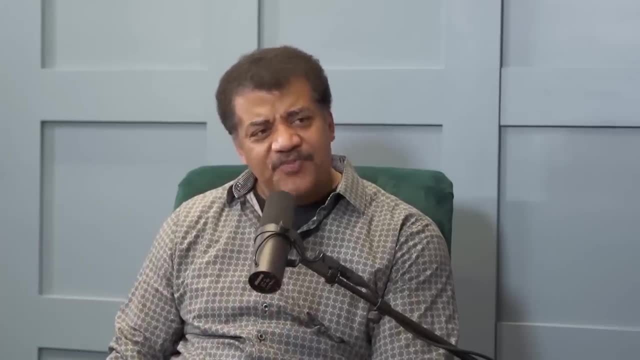 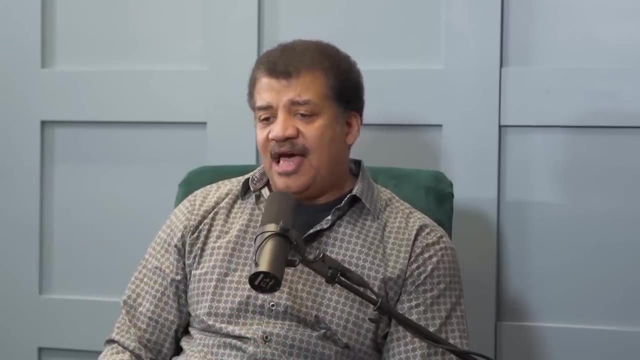 of a sudden, the characters start making sense. It's not really any different from that, And too many people think that they got to know something instantly in order to ever be good at it. rather than want to achieve something, Go to the Internet and you won't be able to read it. When you get to this point, you have to. 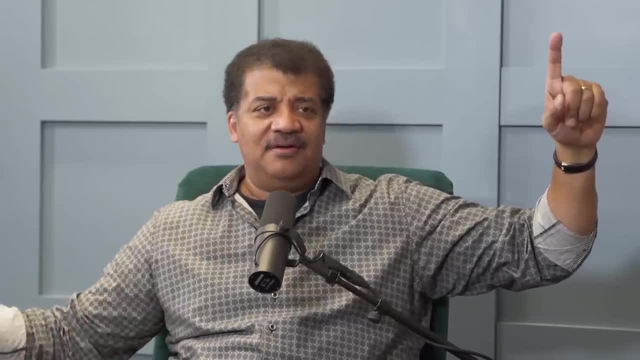 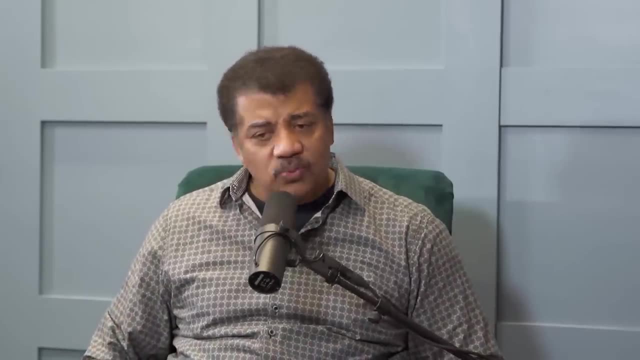 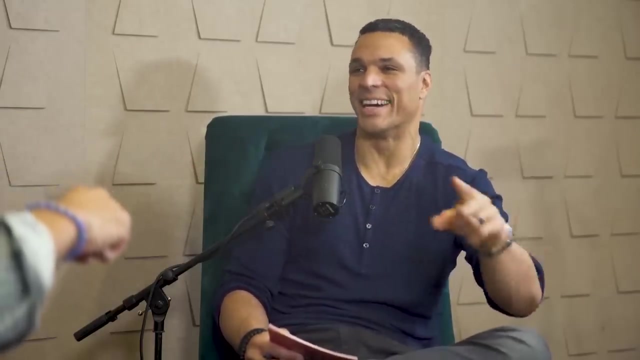 go and try to understand, And I think that this is a real challenge. It's say again: find it and imagine it. If you can find it and realize that there are these hurdles, work at it, And every bit of yourself you invest helps to dissipate that fog And the more badly you want to get there. 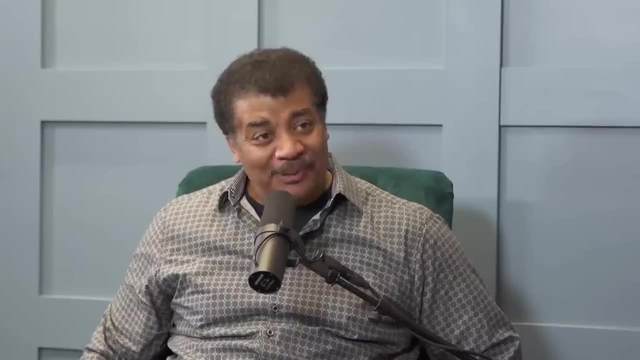 the more you will work to dissipate that fog, And that's what happened to me, And I've invoked that ever since. Yeah, I've been tutored. That's already sounding like my mother. right now She's over there asking for some help.